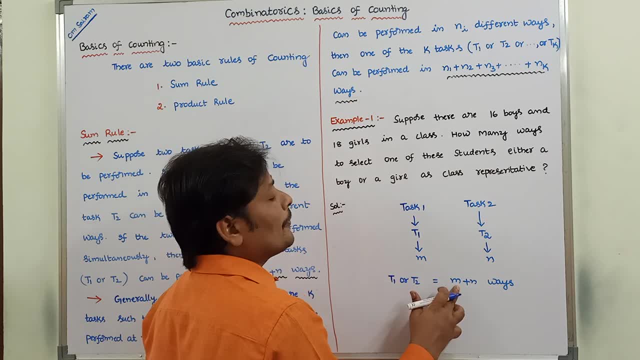 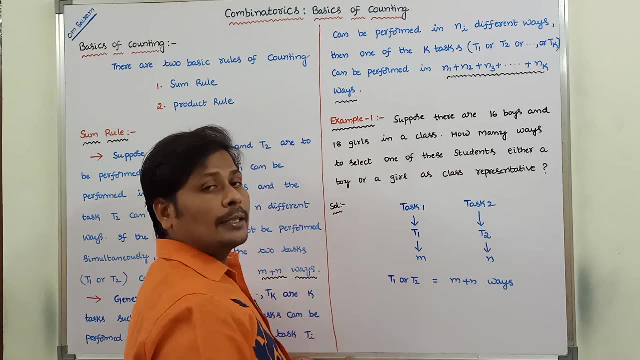 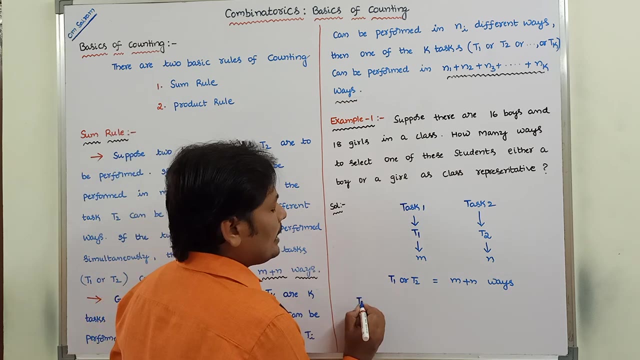 number of ways of performing task T1.. N is nothing but number of ways of performing task T2.. Okay, Next, in general. so there are N tasks. are there? T1, T2, T3, up to Tn tasks are there? Okay, T1 task can be performed in. 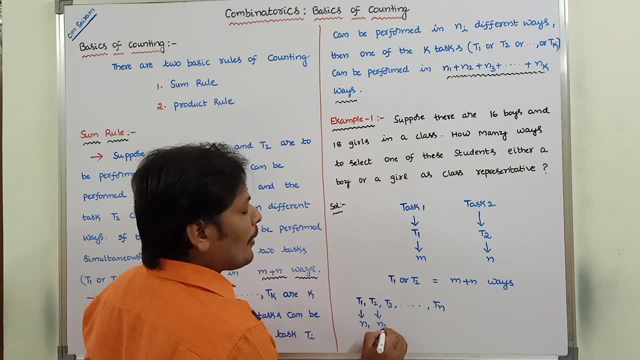 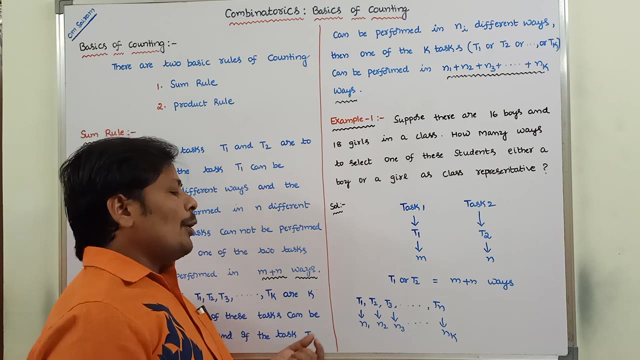 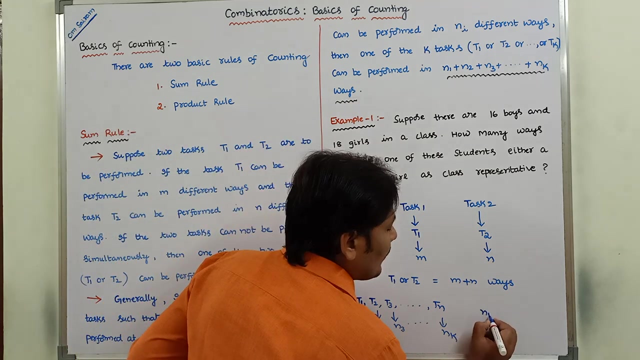 N1 ways and T2 task can be performed in N2 ways. T3 task can be performed in N3 ways and Tn task performed in niños of Its K Ways. Ok, Then one of the n tasks can be performed in n1 plus n2, plus n3 plus up to n sub x k ways. 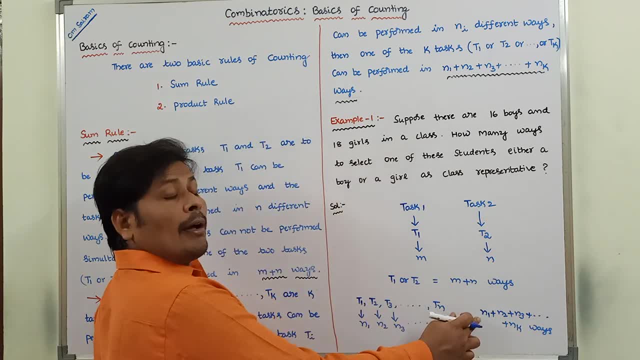 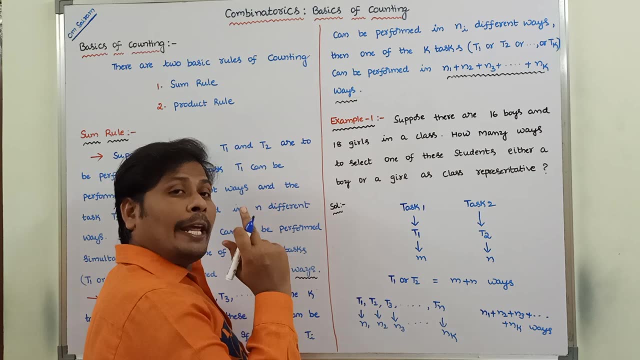 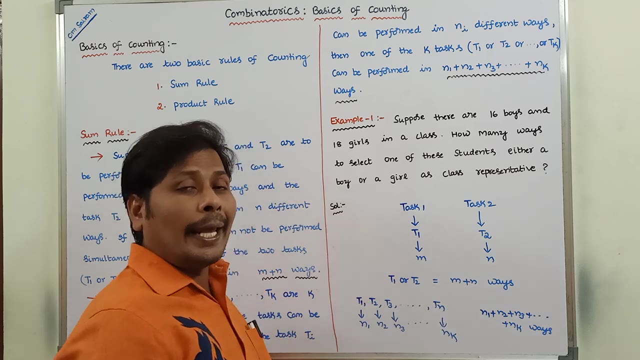 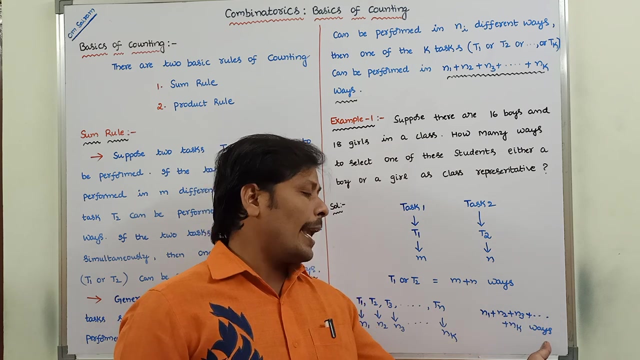 Okay, so this formula is used for finding out among the n number of tasks. Okay, only one task, either t1 or t2, or t3 or tn, can be performed in how many ways. That is n1 plus n2 plus n3 plus up to n sub x k ways. 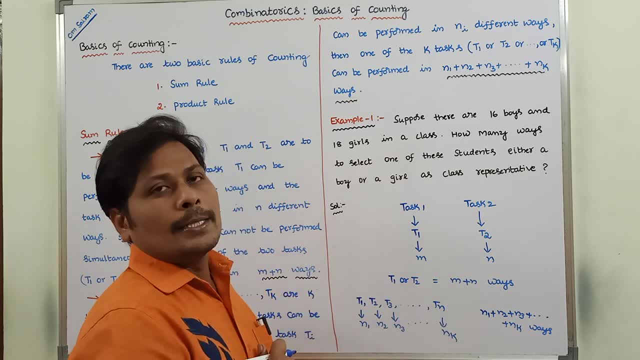 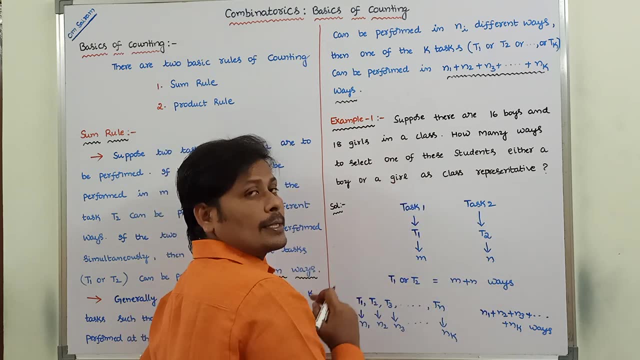 So this is the general rule of the sum rule. Okay, so this is only for two tasks. Okay, this is for n tasks. Okay, two tasks can be performed. T1 task can be performed in n different ways. T2 task can be performed in n different ways. 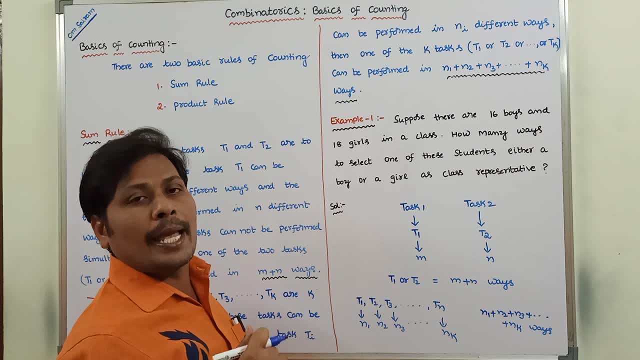 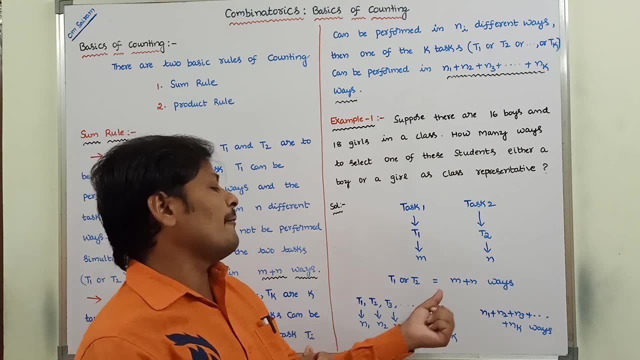 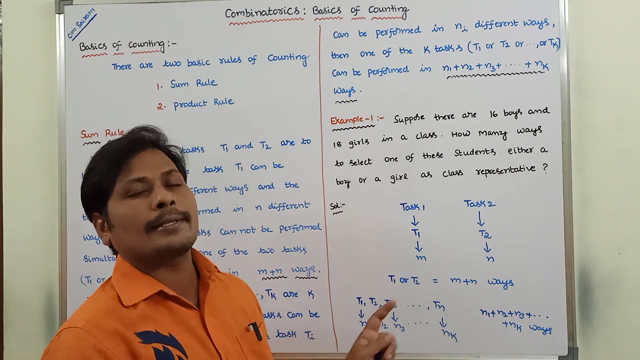 T1 and T2 task cannot be performed simultaneously, Then any one of the two tasks can be performed. in how many ways? That is n plus n ways. Okay, in general there are n number of tasks are performed. So t1 task can be performed in n1 different ways. 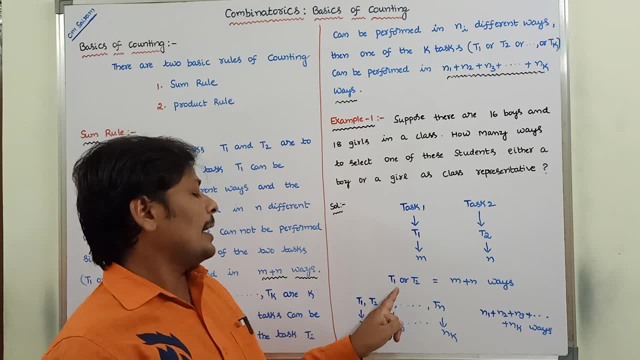 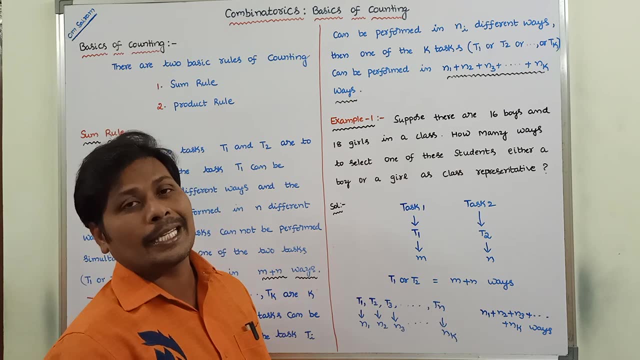 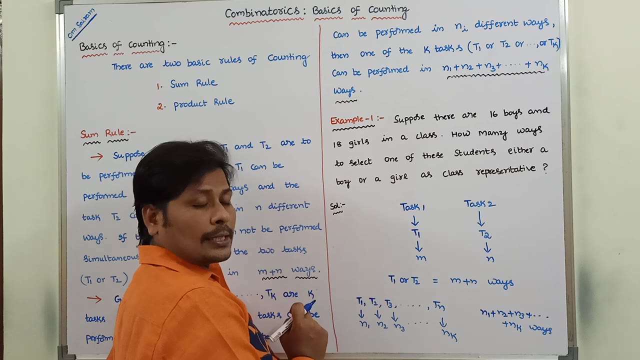 T2 task can be performed in n2 ways, T3 task can be performed in n3 ways And tn task can be performed in n sub x k ways. Okay, so one of the among n number of tasks can be performed in how many ways? 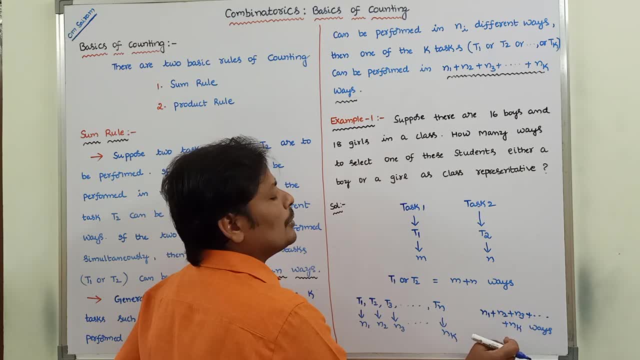 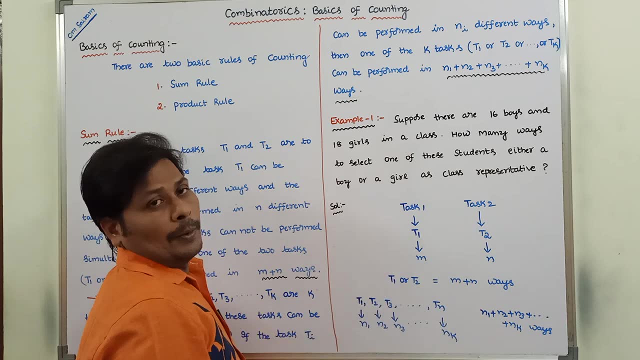 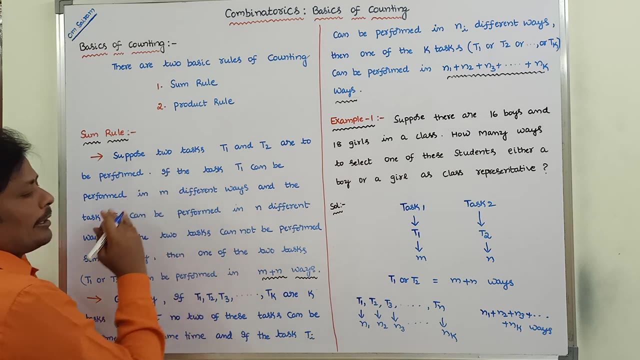 That is n1 plus n2 plus n3 plus up to So n sub x k ways. Okay, so this is the description about the sum rule. Okay, so please check this one, whatever I am discussing, so that we are written as a. 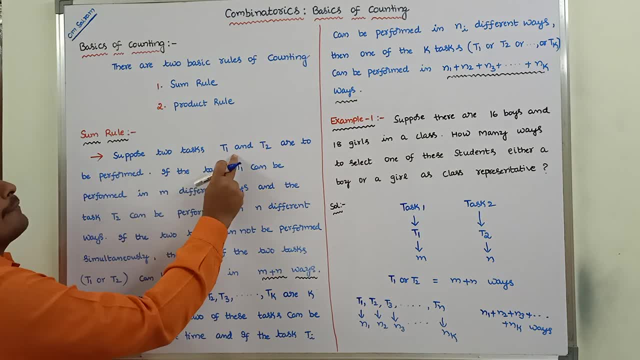 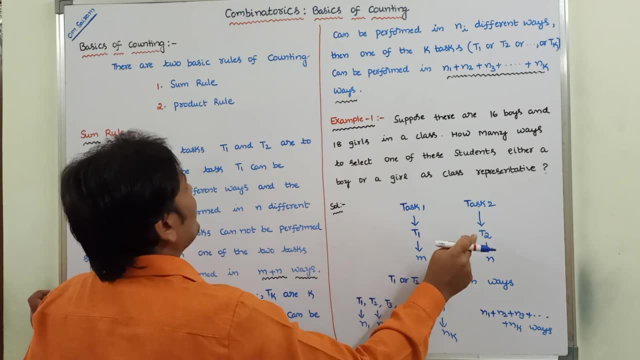 notes. Okay, suppose two tasks, t1 and t2, are to be performed. Suppose two tasks are performed: t1 task and t2 task. If the task t1 performed in n sub x k ways, then t1 task can be performed in n sub x k ways. 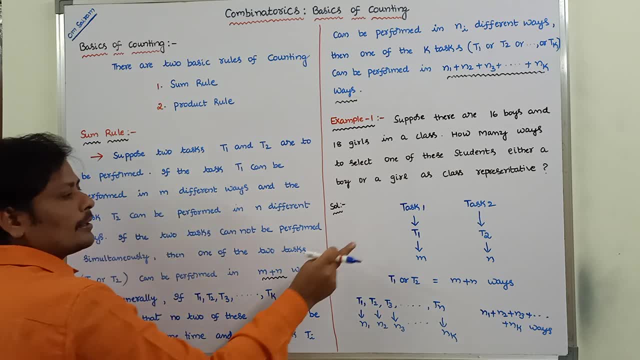 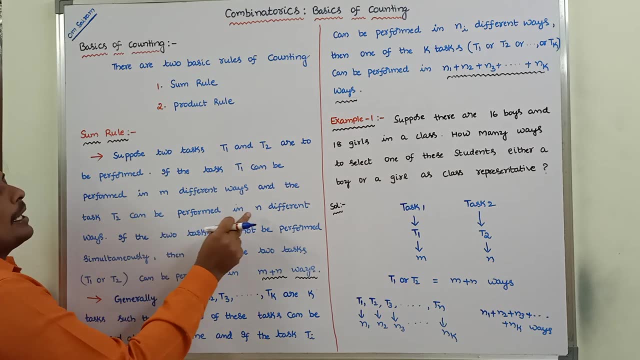 Okay, so this is the description about the sum rule. Okay, so please check this one. All the sub n numbers of tasks can be performed in m different ways. Task t1 can be performed in m different ways, And task t2 can be performed in n sub x k ways. 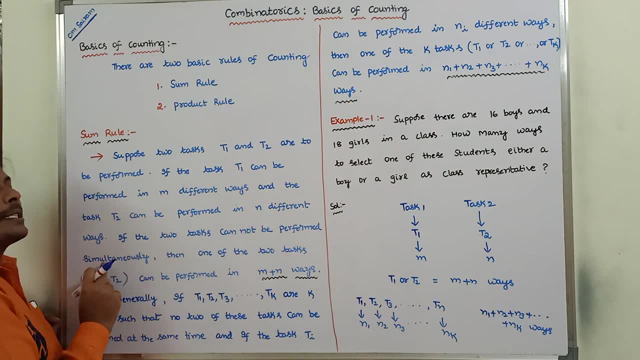 Okay. next, if the two tasks cannot be performed simultaneously, Okay, then one of the two tasks, t1 or t2, can be performed. in how many ways? That is n, sub x, k och ways. Next, one general rule: If there are n, number of tasks, are there or k number of tasks are there, t1, t2, t3, up to tk or k tasks, such that no, two tasks cannot be performed simultaneously? okay, 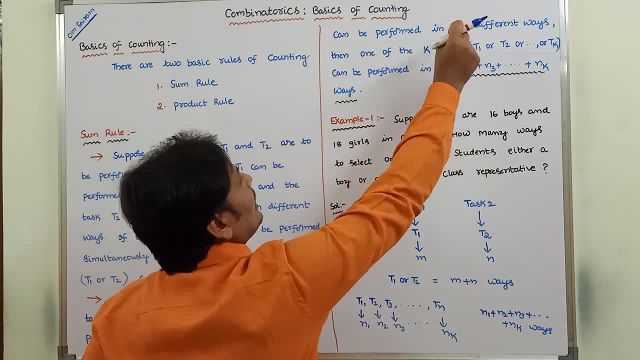 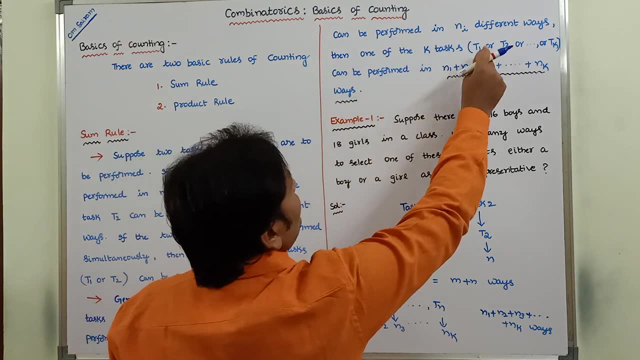 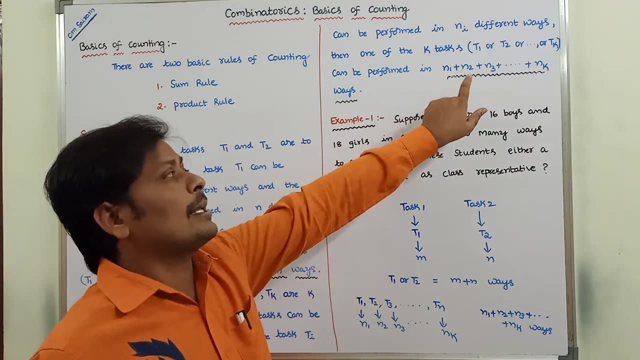 And if the task ti can be performed in n suffix i different ways, okay, Then one of the k tasks, that is, t1 or t2 or t3 or up to tk, can be performed in how many ways? n1 plus n2 plus n3 plus up to n suffix k ways, okay. 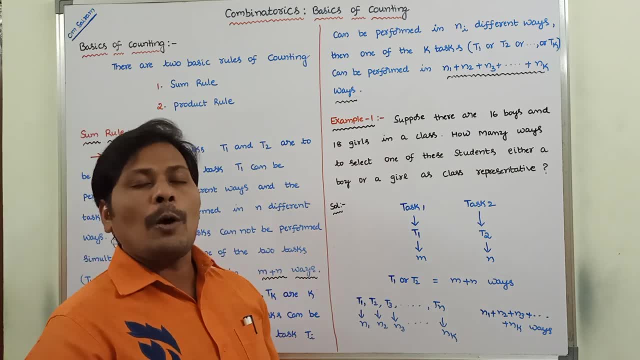 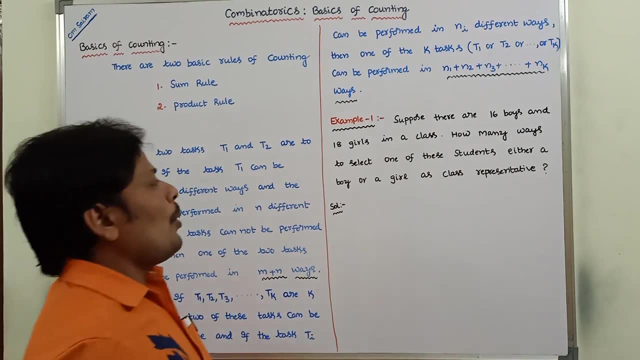 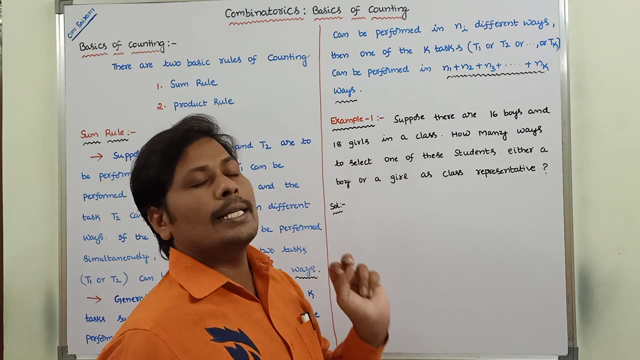 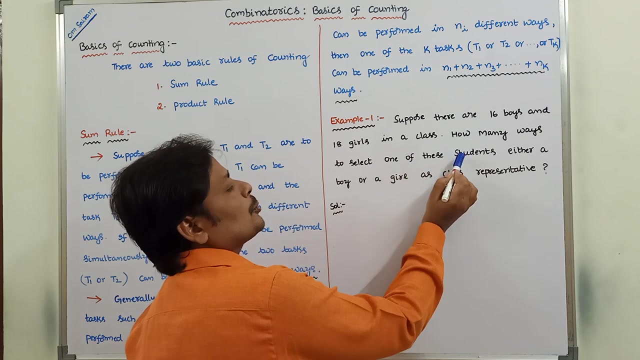 This is the description about the sum rule. Now we can go for some example problems on sum rule. okay, Now we can go for example one problem: Suppose there are 16 boys and 18 girls are there in a class. okay, How many ways to select one of these students, either a boy or a girl, as class representative? 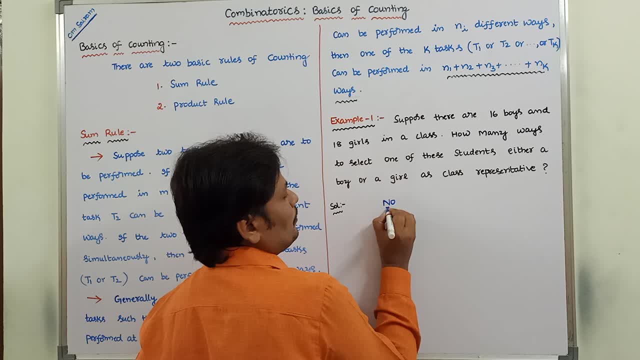 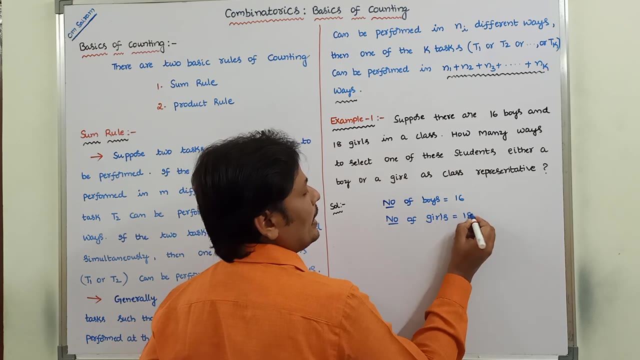 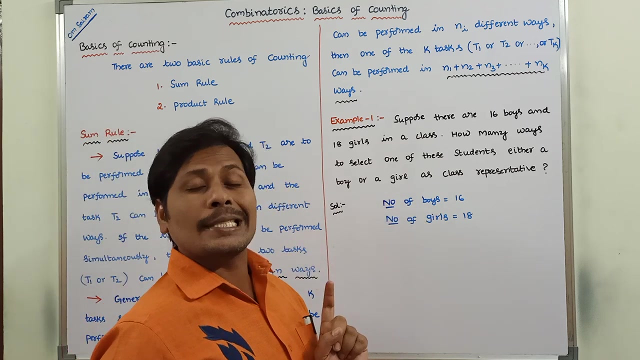 That means so number of boys. so number of boys is equal to 16.. Next, number of girls: Number of boys. Number of girls: Number of girls in a class is equal to 18,. okay, So among the 16 boys, we want to select one boy as a class representative. 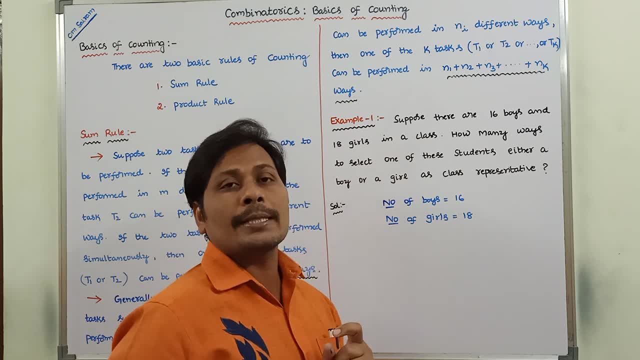 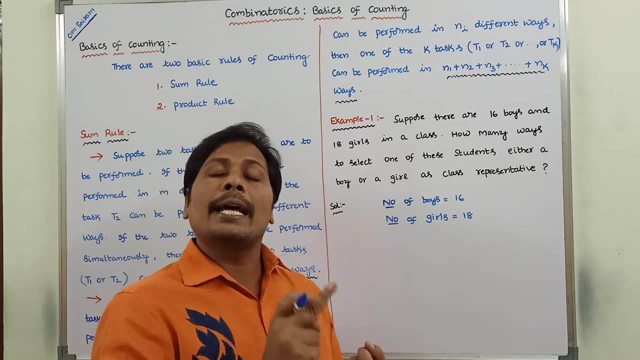 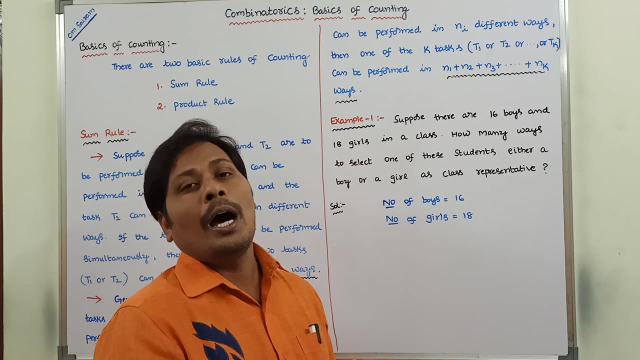 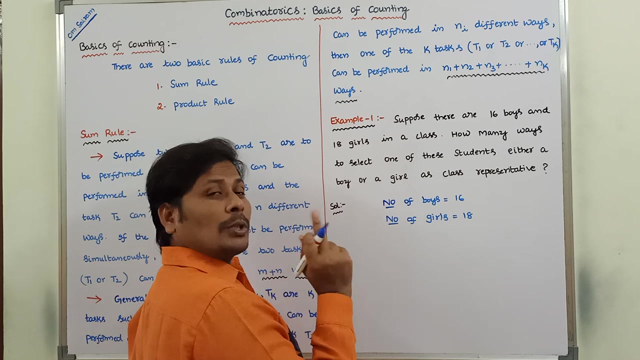 Next, among the 18 girls, we want to select one girl as a class representative. okay. When we are combining, either a boy or a girl can be selected as a class representative. How many number of ways? okay? So here, according to the sum rule, here two tasks are there, okay. 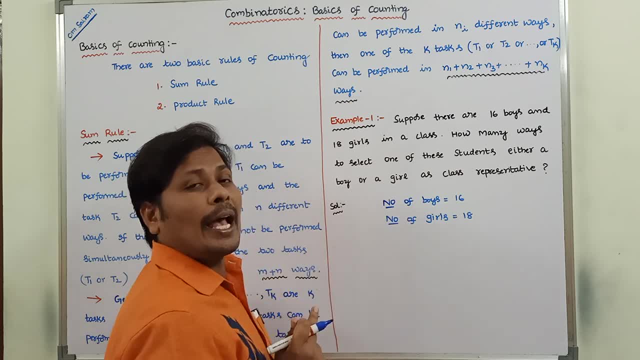 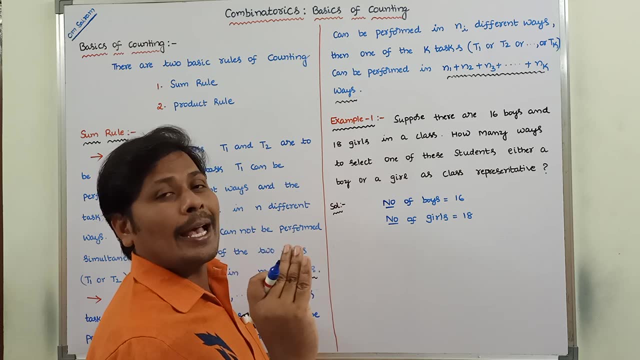 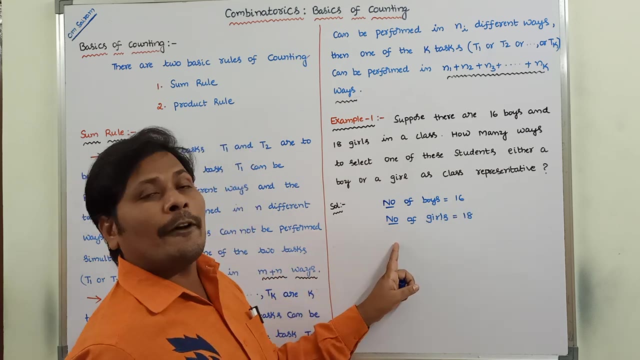 First task means a boy can be selected as a class representative. So how many number of ways of selecting a boy as a class representative? That is 16 ways, okay. Next, how many number of ways a girl can be selected as a class representative. 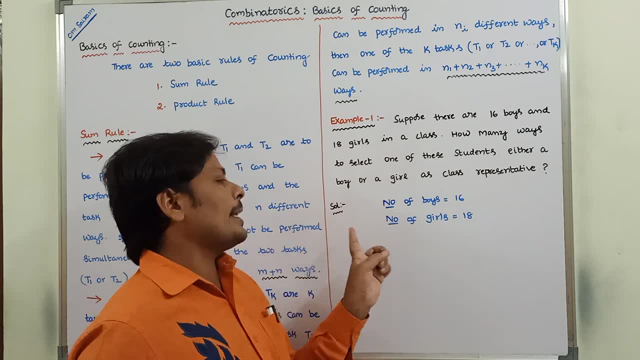 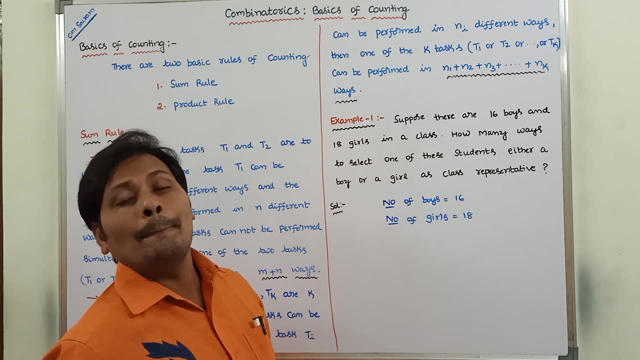 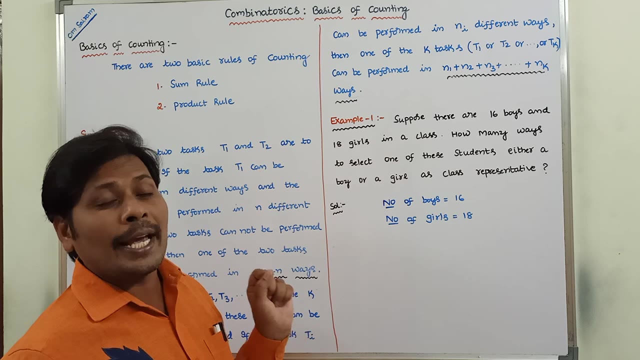 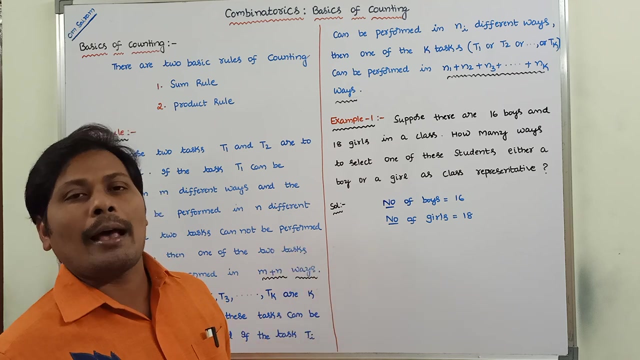 That is 18 ways. okay, Either a boy or a girl can be selected as a class representative is m plus n, That is 16 plus 18, that is equal to 34.. So 34 ways are there for selecting either a boy or a girl acts as a class representative. 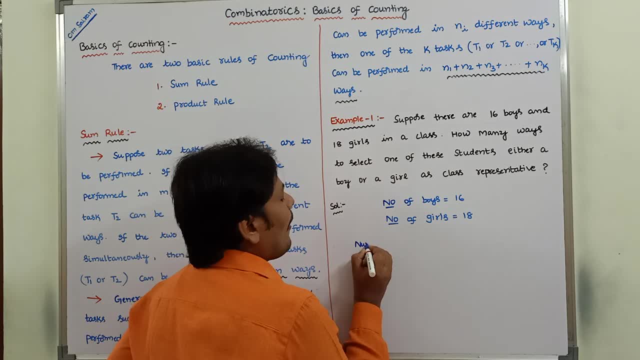 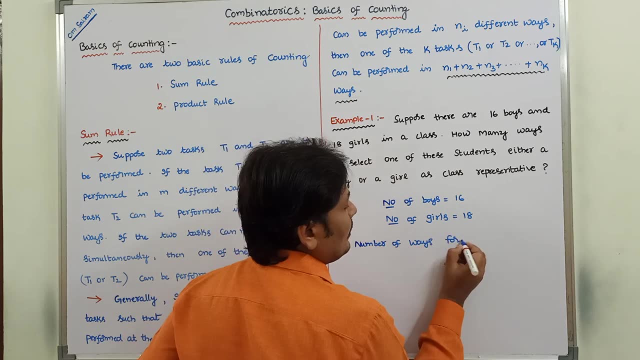 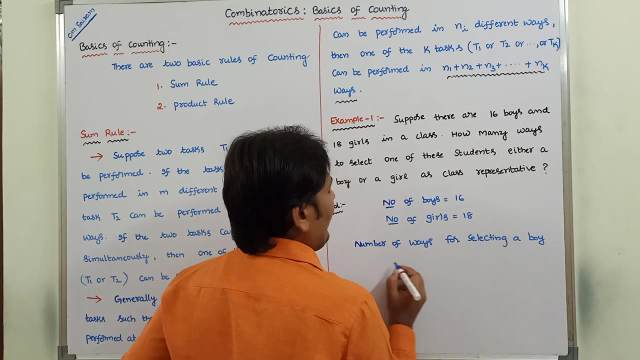 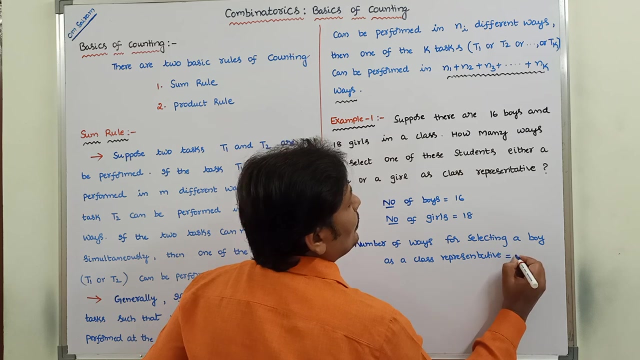 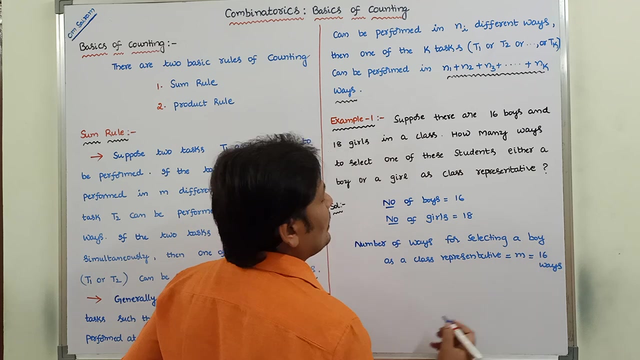 So that means: so number of ways, number of ways for selecting, for selecting a boy as a class representative, as a class representative. So this is task one, okay. Next, how many number of ways is equal to m ways? m ways is nothing but 16 ways, 16 ways, okay. 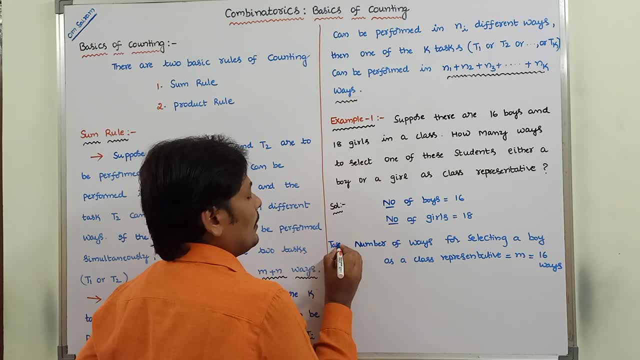 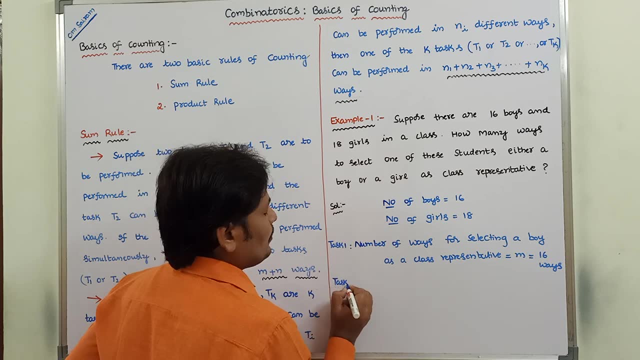 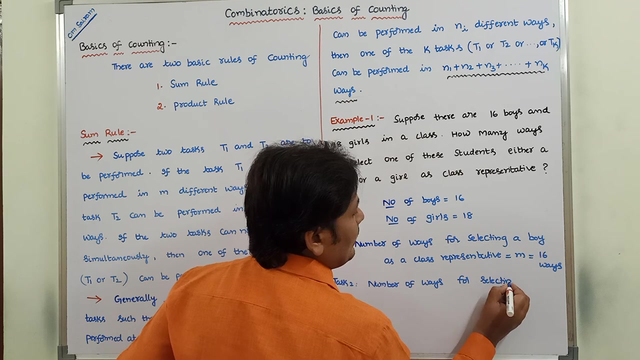 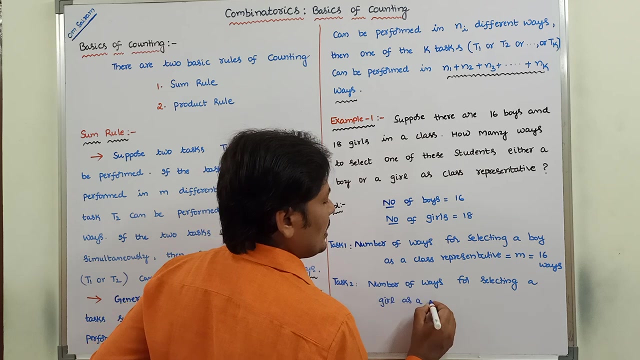 So this is a task one. I am treating this is a task one. okay, Next task two. task two means number of ways, number of ways for selecting a boy or a girl as a class representative. For selecting, for selecting a girl, a girl, as a class representative. class representative. 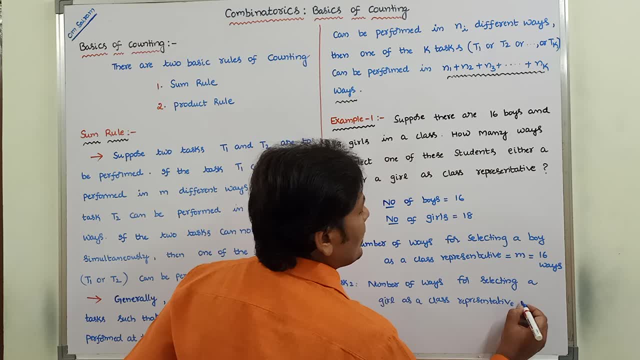 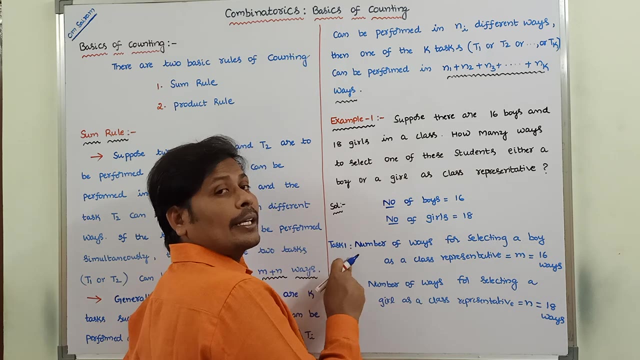 So how many number of ways? so that is a n ways. n is nothing but number of ways. so that is 18 ways. okay, Next one, Next one. So in the task one a boy can be selected as a class representative among the 16 boys. 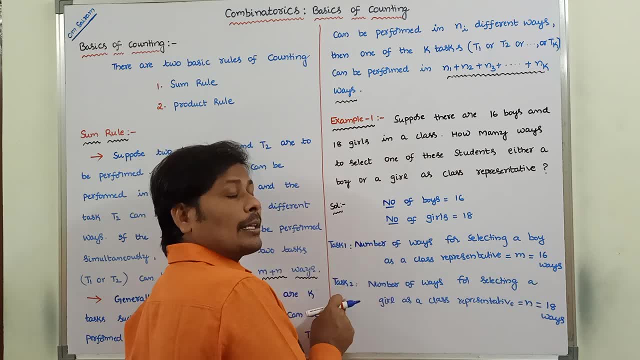 How many number of ways? 16 ways. Next, in task two, how many number of ways for selecting a girl as a class representative? that is n ways. n is nothing but 18 ways. So task one and task two cannot be performed simultaneously. 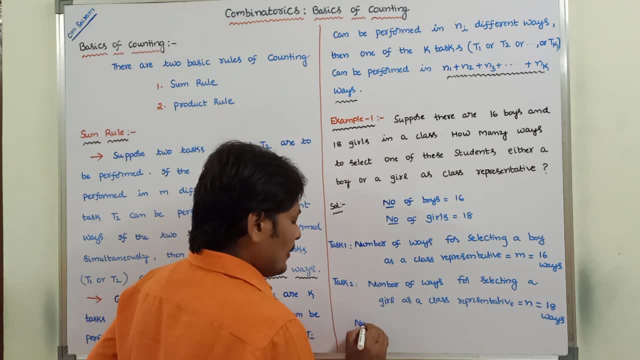 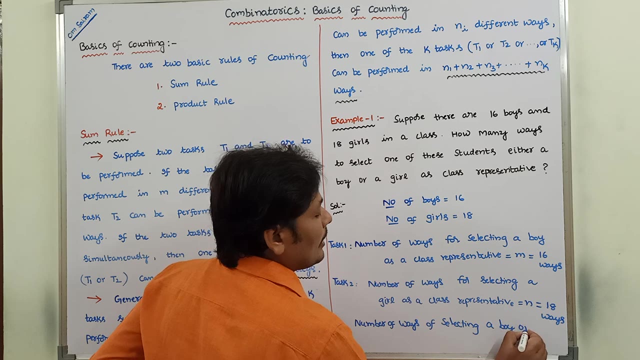 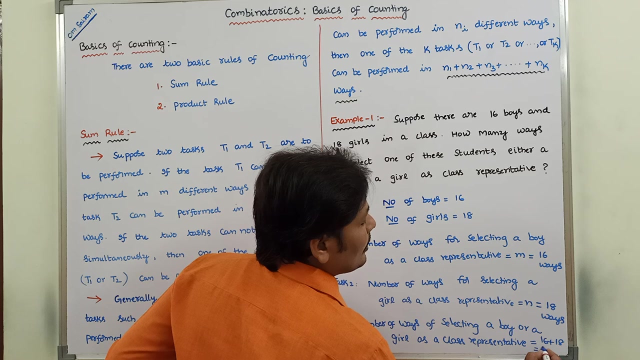 Now. So, number of ways, number of ways, number of ways of selecting. selecting a boy or a girl, a boy or a girl as a class representative. as a class representative, as a class representative, that is equal to 16 ways plus 18 ways. so 16 plus 18, so that is equal to 34 ways. 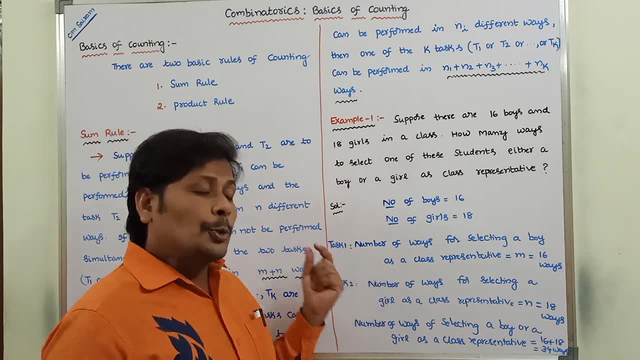 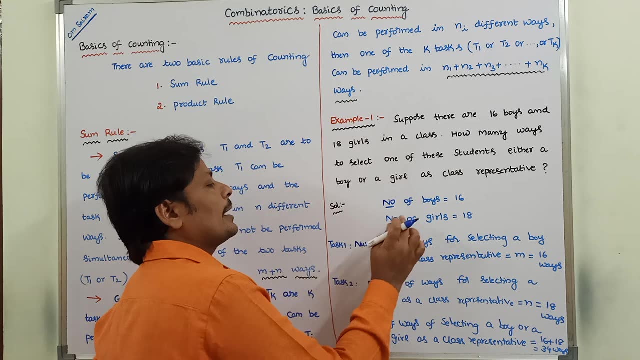 34 ways are there for selecting either a boy or a girl to be acts as a class representative. So here this is a number of. n way is nothing, but number of boys is equal to 16,. number of girls is equal to 16,. 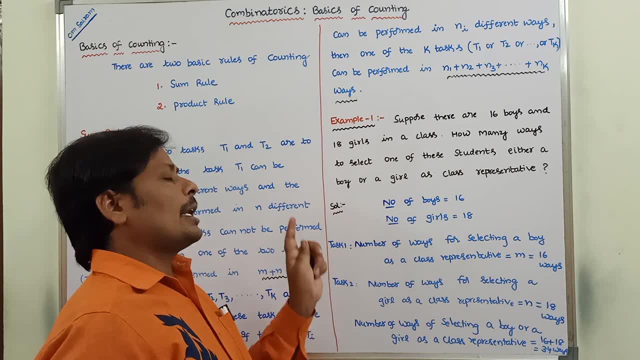 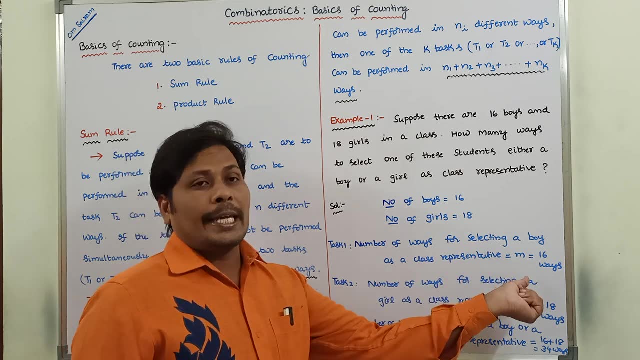 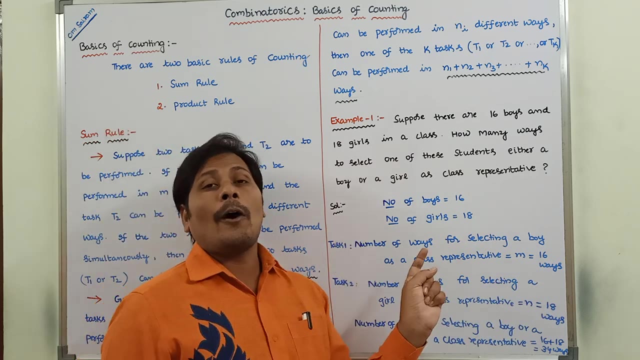 number of girls is equal to 18.. So the number of ways of selecting a boy as a class representative is equal to m ways. m is nothing but 16 ways. This is a task one. Next number of ways of selecting either a girl can be taken as class representative.